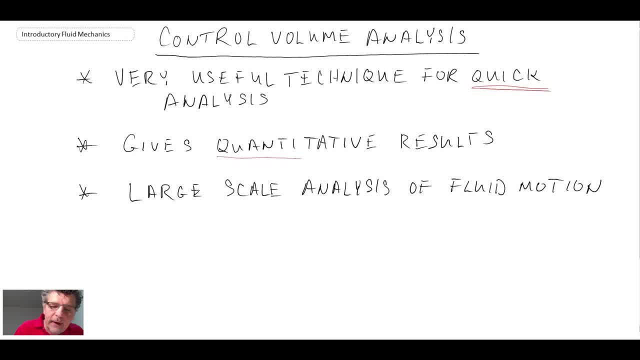 of problems involving fluid flow. We'll be able to get quantitative results out of this, such as forces that might be acting on objects that are immersed in a fluid flow or forces upon a wall, And this is essentially a large-scale analysis, So typically with control volume. 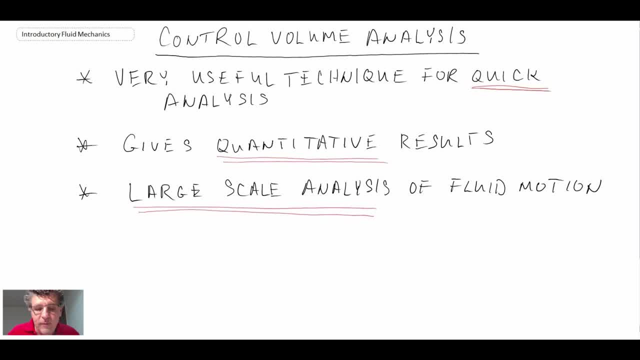 analysis, you're not going to be able to determine specifically what the velocity profile might be on the inlet or exit to a flow field. however, what it is, it gives us these large macro scale values such as drag or lift, based on having measurements of velocity coming into and leaving our control volume. and, in a way, if you think back here, if 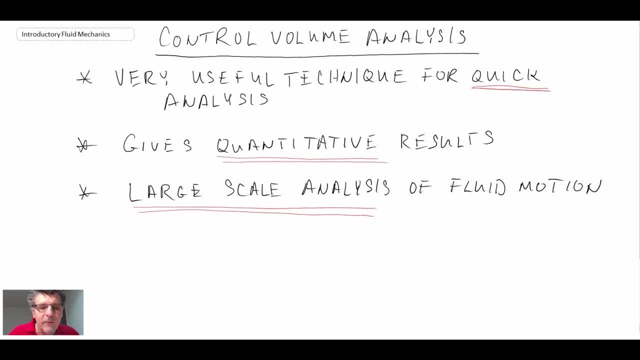 you've taken a course in thermodynamics. in thermodynamics we have fixed mass and we also have the open system and, in certain respects, what we're doing now that the basic equations are always described for a fixed mass- and we'll be talking about that in the next segment- but what we're doing is, uh, formulating our calculations to be able to allow. 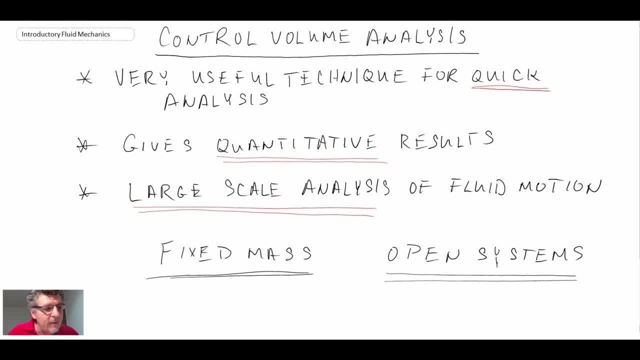 us to do open systems. so we have mass crossing the the boundary and, if you're calling it a from thermodynamics, quite often we use control volumes. we use control volumes and fluid mechanics as well. however, in thermal we mainly focus on the energy equation. here we can look at the momentum. 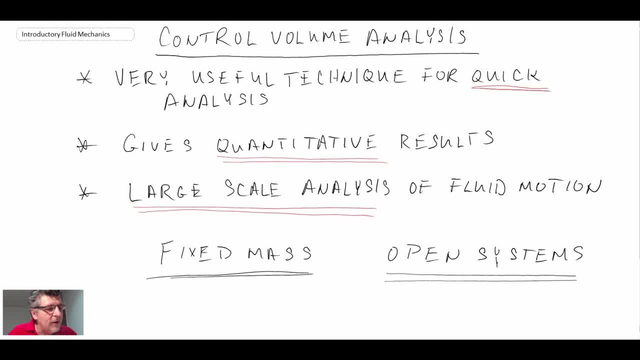 equation, a linear angular. we can look at mass conservation, we also look at energy, so we kind of expand the portfolio of things we look at when we're doing fluid mechanic analysis. but it is very similar to what we do in thermodynamics. so, to begin with, what is a control volume? and? and so i 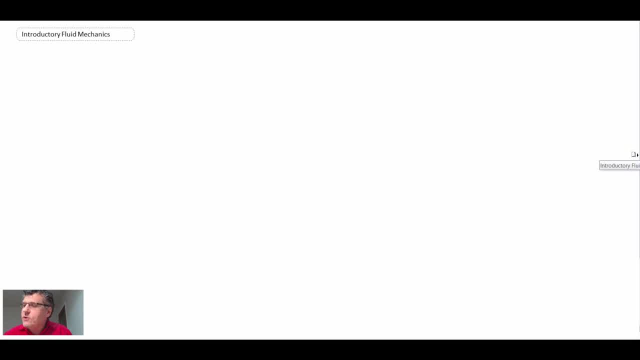 want to take a quick look at what a control volume is before we get into the details of deriving the equations for the control volume. so let's take a look at an example: control volume, and sometimes what you'll see me do is something like this: that is an abbreviation. 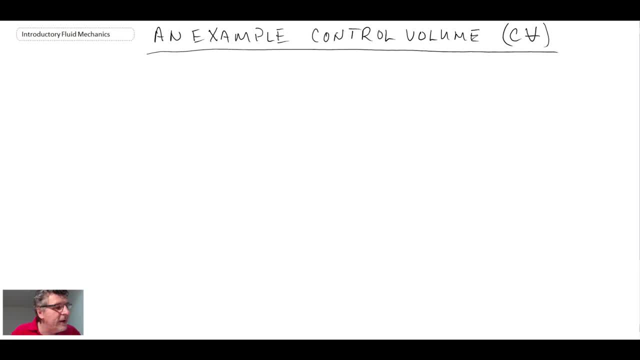 for control volume, cv, with a line there through it. so let's take a look at something that we can all relate to. let's say we have a jet, so we have a flow. it could be a garden hose nozzle or something like that, but it would accelerate the fluid coming through it, and so let's say this is all solid. 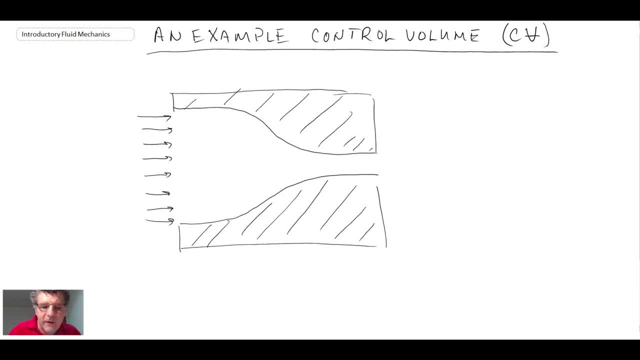 and let's say we have a uniform velocity profile coming in. chances are you wouldn't, but you may condition the flow to give you something like that. so that's v in and then on the outlet because the area is contracting. let's say this is a liquid, so it's incompressible. 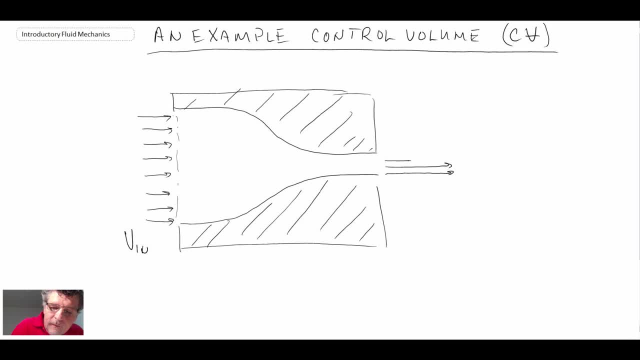 the velocity is going to increase and that would be v out. so if we were to do control volume analysis of this, where you sketch your control volume analysis, you would have to do a control volume analysis of this and then you'd control volume is quite often important for doing the calculations. but an example for this: if you were 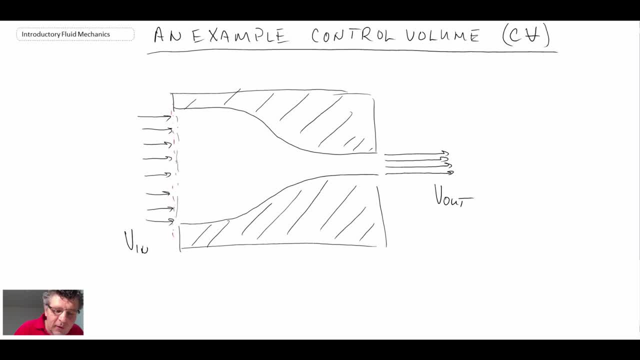 to do control volume analysis. maybe you would decide to put the control volume around the outside of the block itself, and so that's what we would have for the control volume, and you'll see then we would do something like this to denote that that is the control volume. another thing is that we have surfaces. 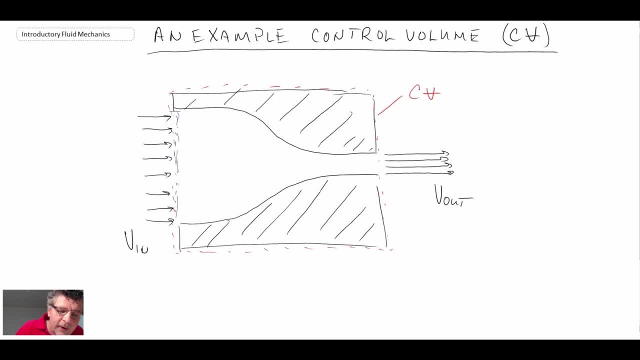 where mass is crossing the boundary. so we have one on the inlet and one on the exit and sometimes we'll write control surface one and maybe control surface two just to denote the fact that that's where the mass is crossing the boundary. so with a control volume, fluid can cross the boundaries. but 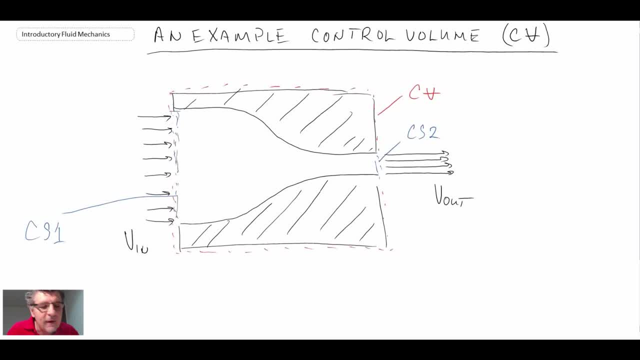 our governing equations are for fixed chunks of mass and consequently we need a way to be able to relate that. so the idea with the control volume is that you only are worried about the boundaries, the inlets and the exits and we don't have to keep track of all of the particles of fluid going through it.